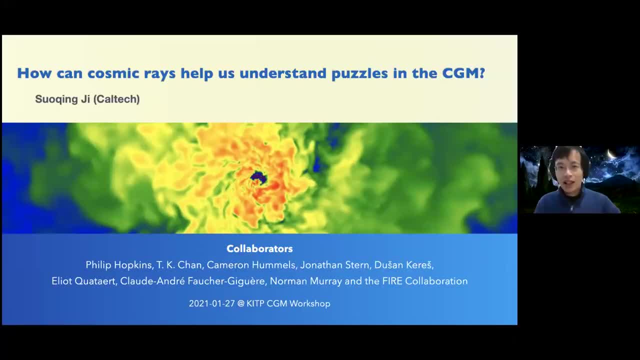 For this, Hey. so good morning everyone. So I'd like to first thank the organizers for organizing such a great workshop, And in my talk I'd like to focus on the impact of custom rates on the CGM And I'd like to argue that maybe, if we bring custom rates, 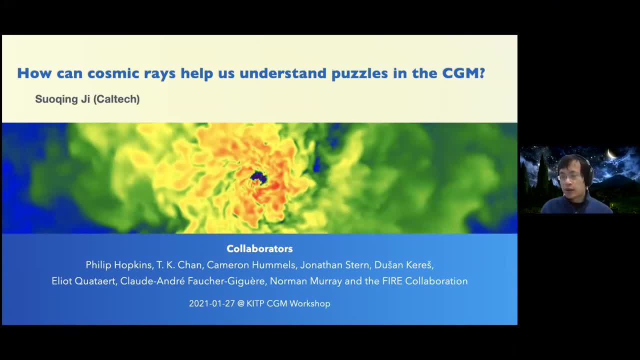 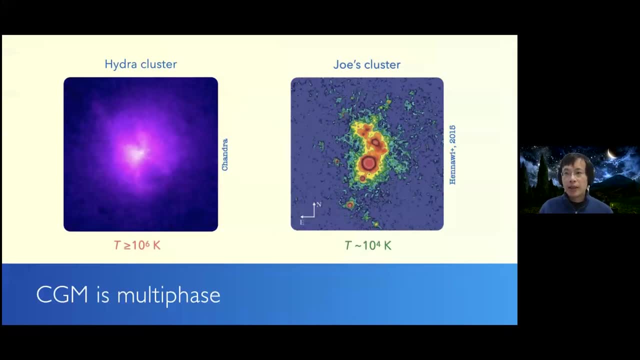 into consideration, we may potentially understand some problems in the CGM. So now we know that the CGM is a multiphase right, So it contains the hot gas above 10 to the fifth Kelvin And also it contains the cool gas at around 10 to the fourth. 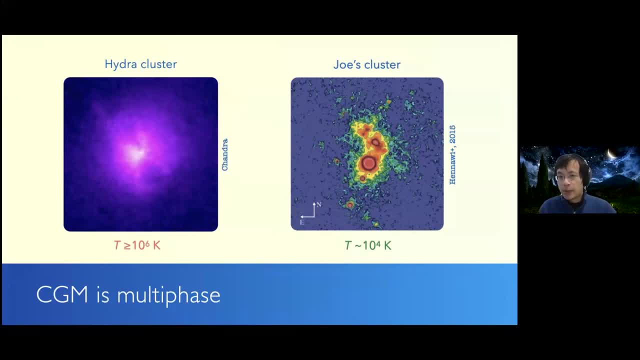 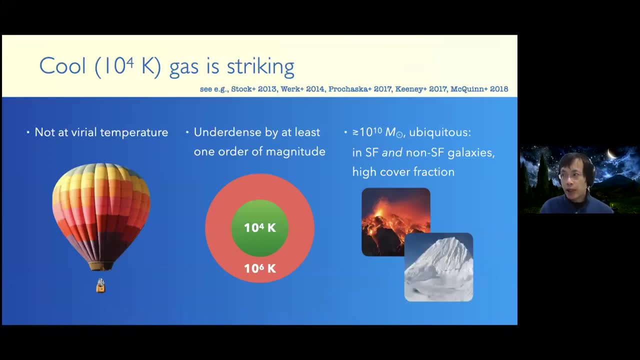 Kelvin. So that's indicated by the emission and also absorption. And if we consider the cool gas, or let's say the cool gas is striking, why is that So? first of all the cool gas, the temperature, and not at the river temperature. 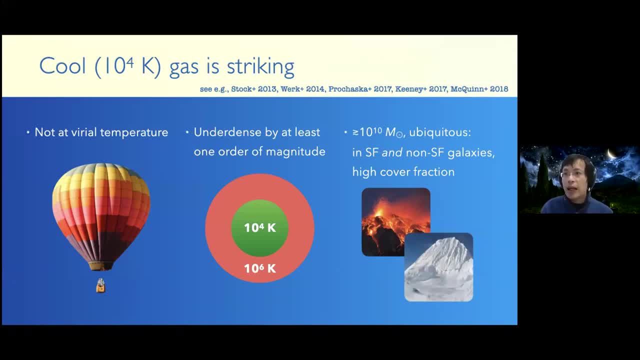 we know that the gas need to maintain a high temperature. Therefore they can have high pressure to support themselves against gravity. Otherwise they will fall into the central galaxy and can not remain at a very large radii, just like the balloon here, right. 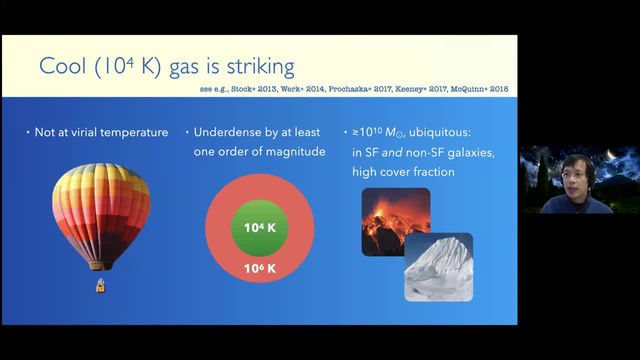 You know, the balloon need to remain hot to float in the sky, Otherwise it will sink. But now we know that the gas is only 10 to the fourth Kelvin. that is way below the river temperature. So how can it stay at a very large radii? 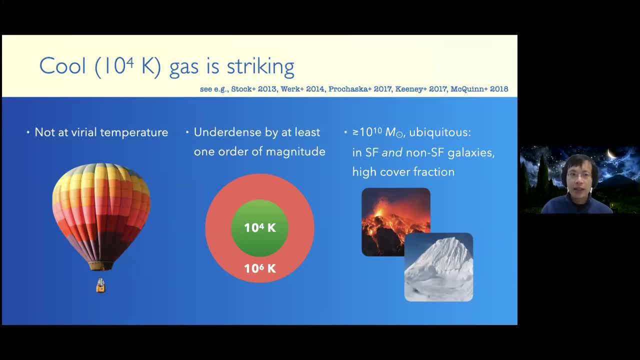 Instead of falling into the center of the galaxy. right? So that is the part of one. The part two is that people find that the cool gas and hot gas they're not in pressure equilibrium. The density of the cool gas is at least one order. 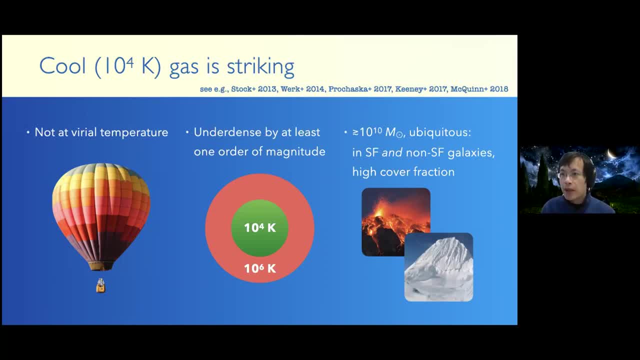 of magnitude smaller than the value required to maintain pressure equilibrium with the hot gas, Which means that maybe the hot gas will try to push the cool gas or try to squeeze the cool gas And cool gas will not be stable right. So the part two is that 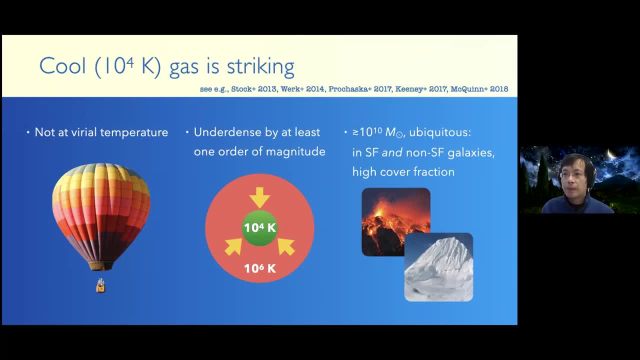 so if the cool gas is under pressure, so how can it be stable, right? So the second part of The third thing is that there's a lot of cool gas. So in your Milky Way galaxy it's at least 10 to the 10th solar mass. 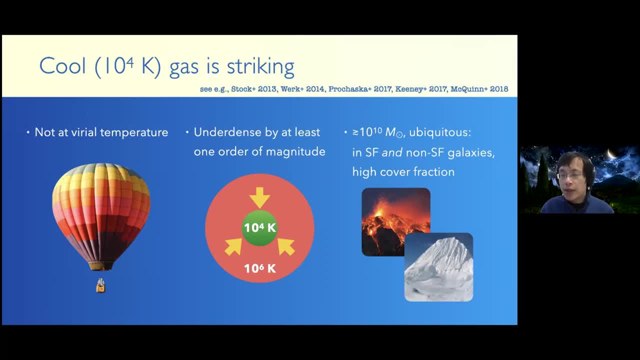 And you can find cool gas in both star forming around non-star forming galaxies and has a very high coefficient. So previously we think that, okay, it can't be hot because there's all the feedback process to heat it up, But actually when we see it, it's cool. 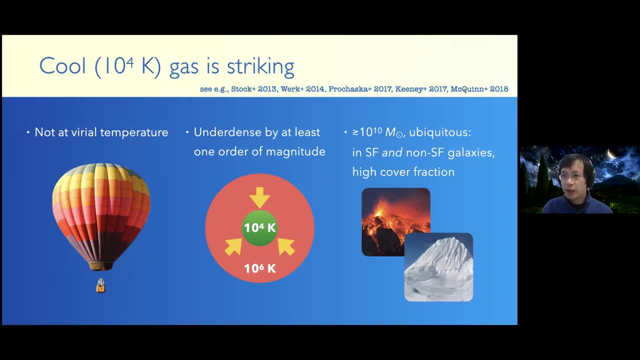 Something like that. we want to see lava here, But actually what we see is snow, and the snow and lava can coexist. So I do think that the cool gas is indeed striking, And also have chatted a lot about O6, right. 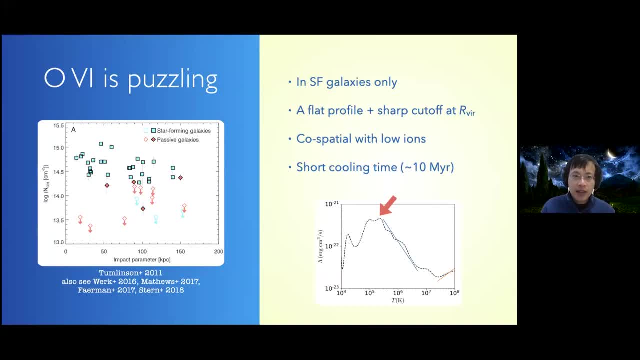 So a long standing problem, And of course, it is positive too. The first thing is that we know that the O6 only can only be found around star forming gases, but not in non-star forming gases, And also we know that the O6 has a very flat profile. 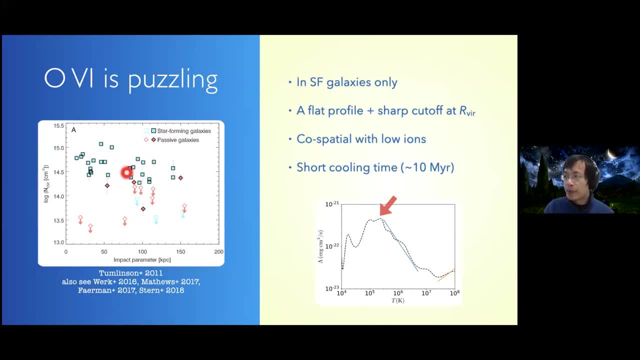 It does not decrease with the increase of the radii right. The third thing is that is O6 is kind of co-spatial with the low ions. So if we say that low O6 trace the warm gas, so why the warm gas always stay together with the cool gas? 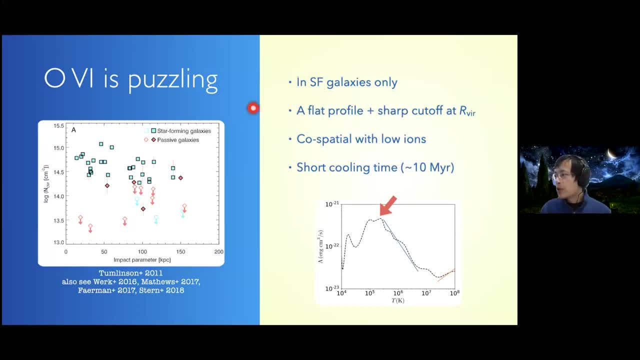 And finally, we know that the O6, corresponding to temperature and the temperature of the O6, has a temperature of three times the fifth Kelvin. So that is, that sits at peak of the cooling curve, So it corresponds to very short cooling time. 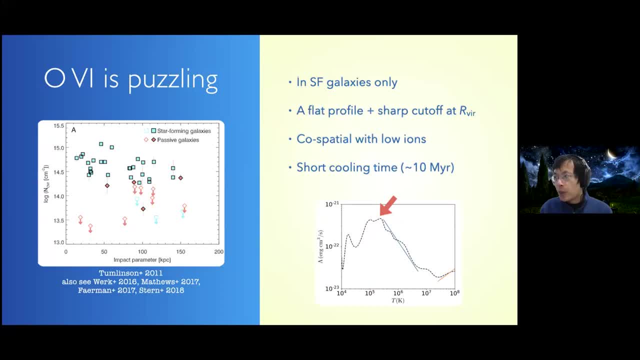 which means that, if this is true, the warm gas will quickly cool down to 10 to four Kelvin And therefore we should not see any warm gas at all. But even given such a short cooling time, so why we can still see a lot of O6 around star forming gases. 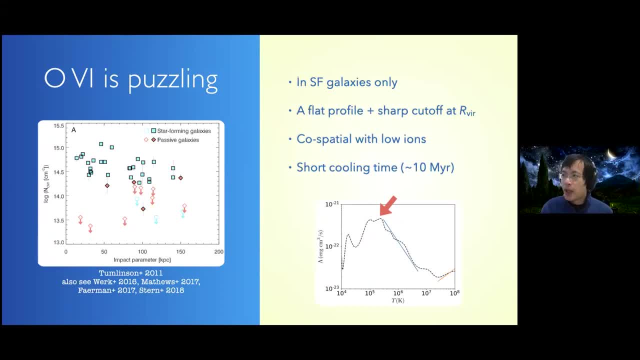 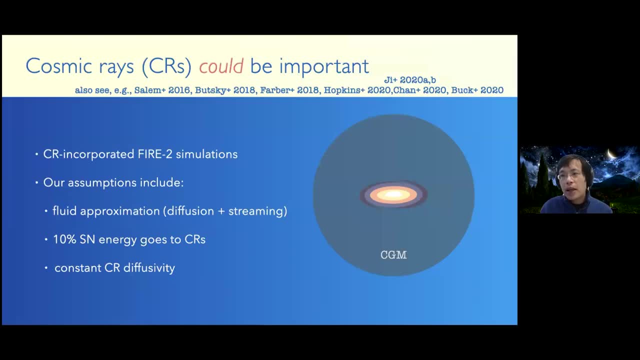 So I think these are the puzzles in the CGM. So that really puzzles me a lot. So in this talk I would like to try to argue that maybe if we include the cost rates and this problem could be resolved, And here I say the cost rate could be important. 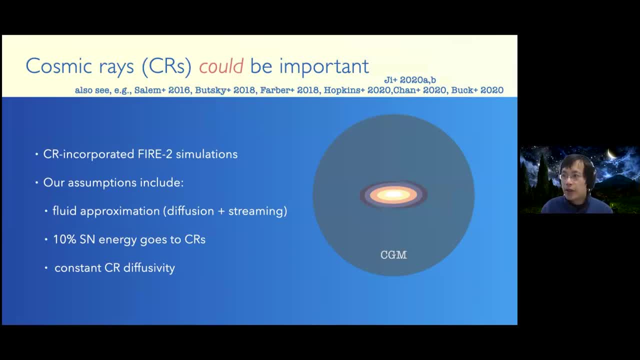 The could means that because we have a lot of assumptions, for example, which we simply concentrate not as particles but as fluids, and we assume that it has some diffusion and streaming, So it really kind of the model dependent stuff. So I say the cost rate could be important. 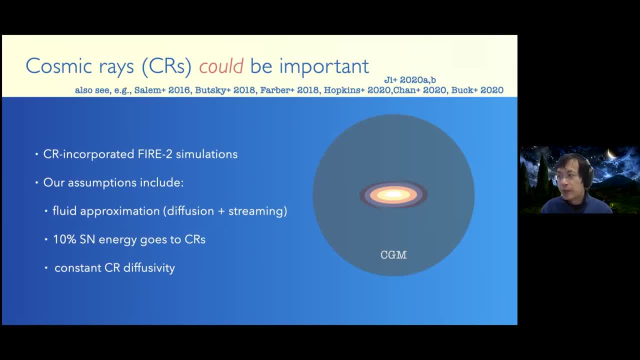 So if this assumption is not too far away from the reality, The best idea is that because we have a supernova explosion in the center galaxy and that we'll try to have some energy input output And the 10% of energy will be converted in cost rate. 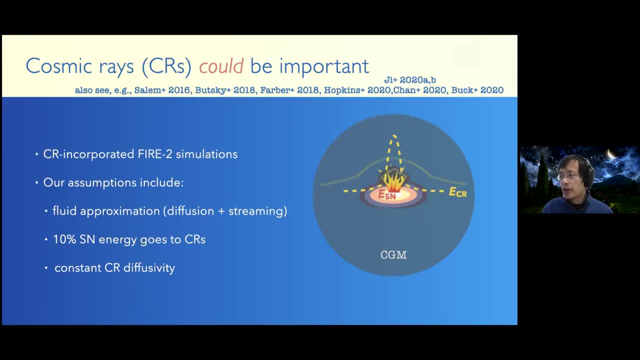 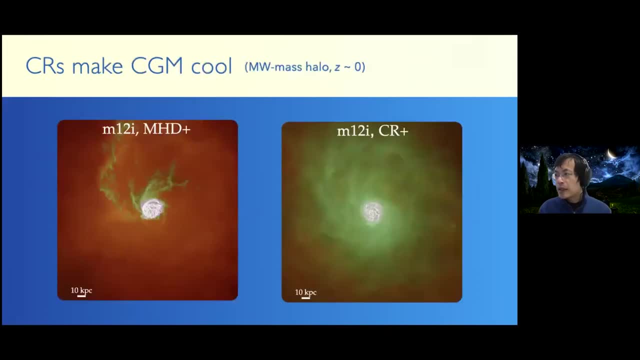 The cost rate can diffuse, diffuse and stream into the CGN so it can build a profile on the CGN. So that is a basic model. So this is the first glance of the simulation, with and without custom array, Left side. the MH50 plus means that it can see everything. 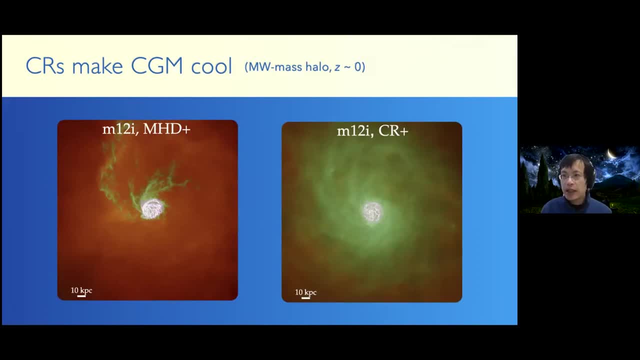 the magnetic fields, viscosity conduction, everything except for custom array And the right hand side. the CR plus means that it is identical to the left-hand side and the only difference is that it contains custom array. So this is apple to apple comparison. 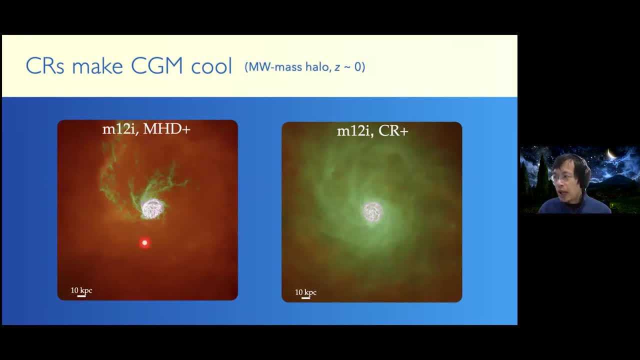 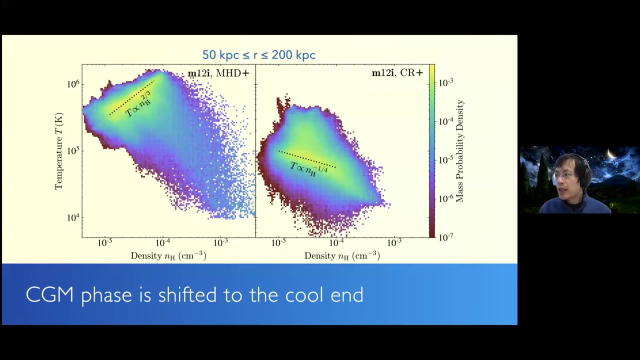 And you can find that without custom array, the entire halo is really hot, right, But with custom arrays the halo become really cool. So that is a huge impact. And if we look at this more quantitatively, you can find that without custom array, 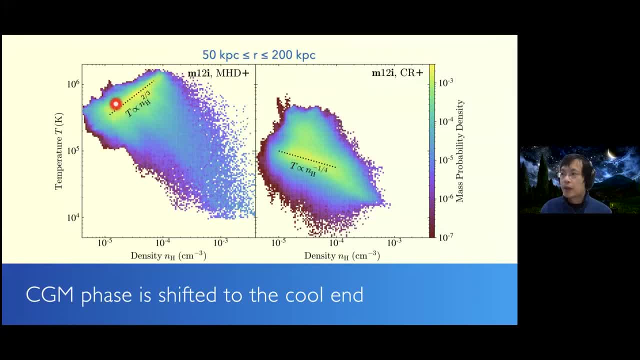 most gas stay above temperature 10 to the fifth Kelvin, so in the warm and hot regime. But with custom array most of the gas stays below 10 to the fifth Kelvin. So it seems that the custom array can have a huge impact on the phases of the CGN. 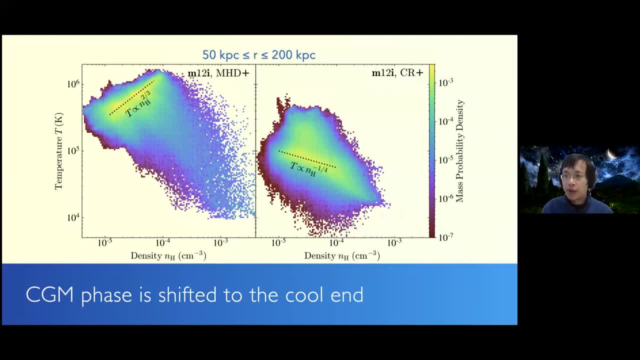 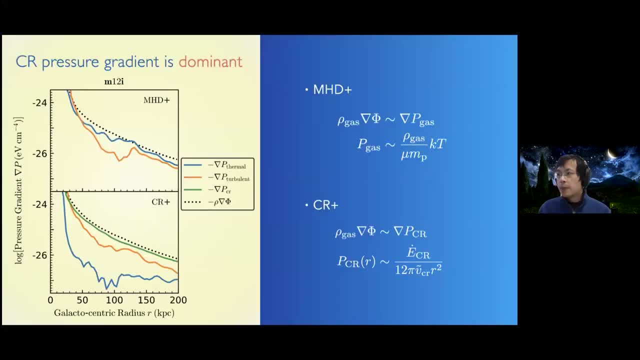 You can shift the phase of CGN from the hot end to the cool end. So am I wondering, why is that? So we can look at the pressure gradient profile and the function of the radius, So here on the top panel. so there's no custom array. 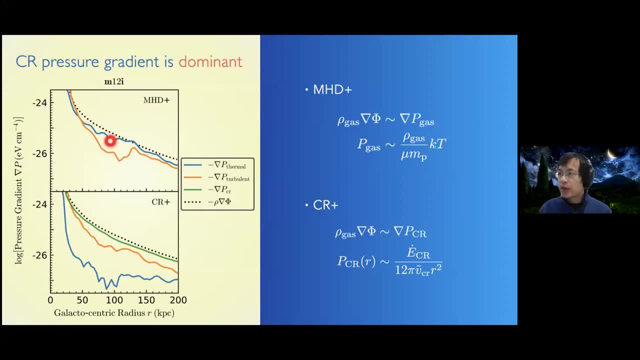 And if you look at the blue curve, that is the thermal pressure, So that is comparable with the black dotted curve. So that is the gravity potential, right. So which means that if there's no custom array, the gas need to remain hot. 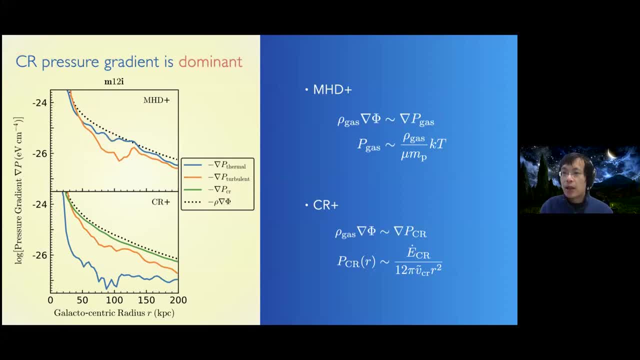 so it can have a high enough pressure to play against gravity, right? So that is our naive thoughts. So, because you can see that the gas need to have a high temperature, because so it can have high pressure so it can bend against gravity. 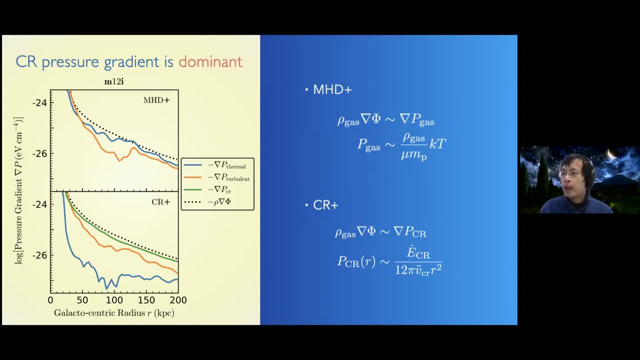 So there's no way the gas must be hot. But now, if we include custom arrays, you can see that the blue curve, that is the gas thermal pressure, becomes at most two orders of magnitude lower, And instead that is the green curve. 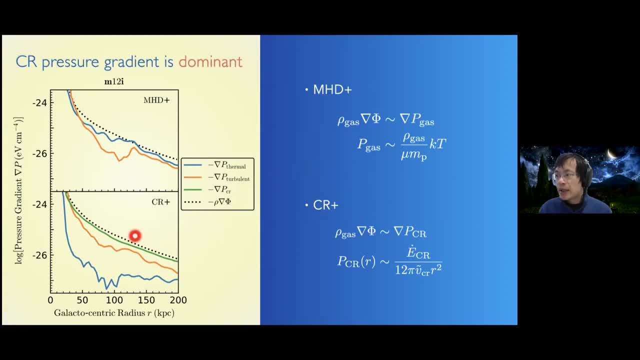 that is the pressure of custom array. that is comparable with gravity. So if the halo becomes custom array dominated then the gas can be supported by custom pressure And we know that the custom pressure will be proportional to the custom array velocity over some stream. velocity of custom arrays. 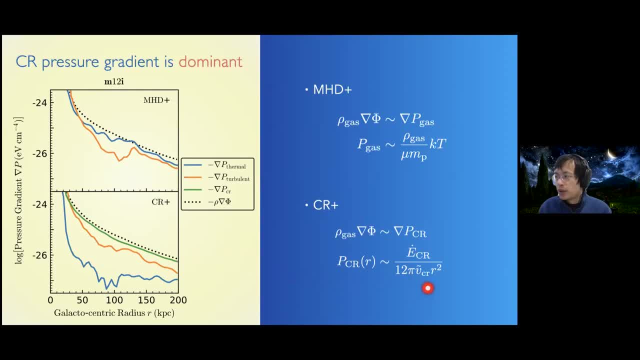 Now. so the radius of the square, of the radius of custom array velocity, right, And that is independent of the gas temperature. Therefore, if we rely on custom array pressure to support a gas, then the gas does not need to be hot anymore. 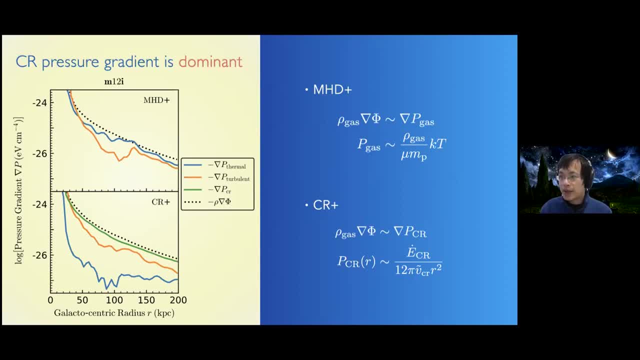 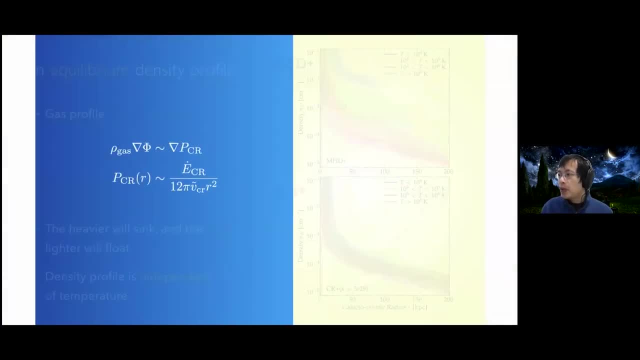 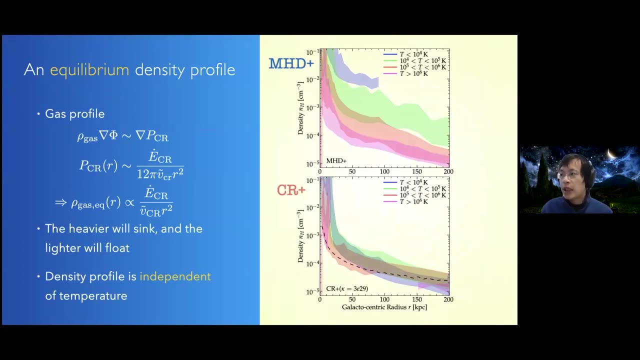 and it can be very cool. So that is the biggest difference with and without custom array. And if we can put these two questions together, we can solve for a density profile. It's so-called the equilibrium density profile. So what does the equilibrium word mean? 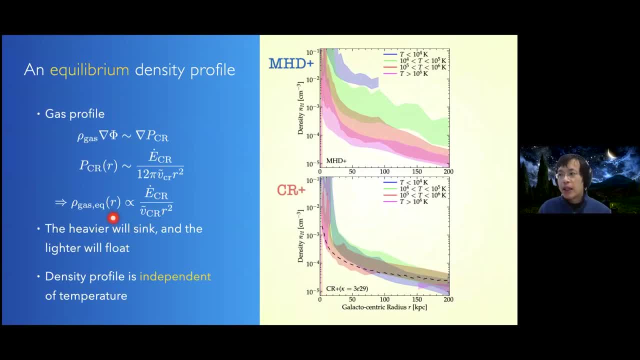 So it means that, as some radius are, if the local density is greater than this equilibrium density profile, then locally there will not be enough customer pressure to support it, So it must sink right. So, on the contrary, as the radius are, 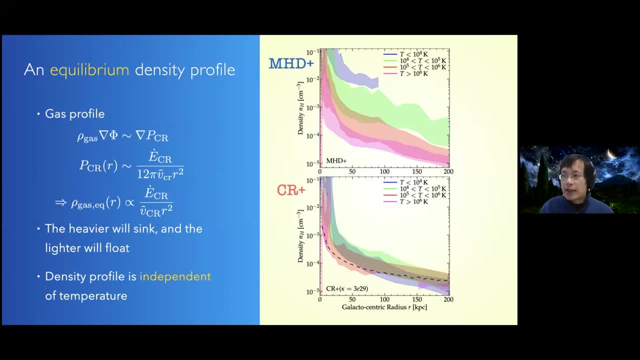 if the density of the gas is smaller than this equilibrium density profile, then locally there will be too much customer pressure to support it, to act on it, So the gas must float. So in other words, only when the gas density equals this equilibrium density profile. 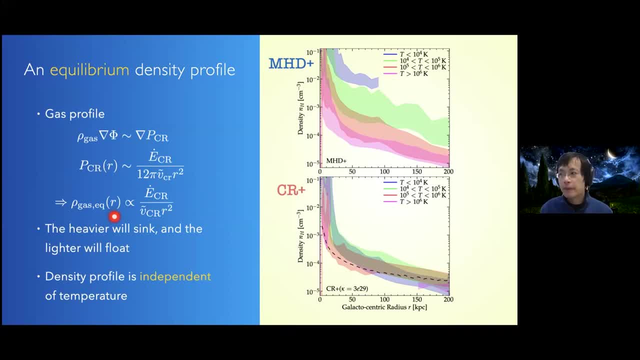 as the radius are, the gas can survive right And you can find that this density is independent of the temperature. That's very important And that is exactly what we see from our simulations. So on the top part. so here I show the gas of. 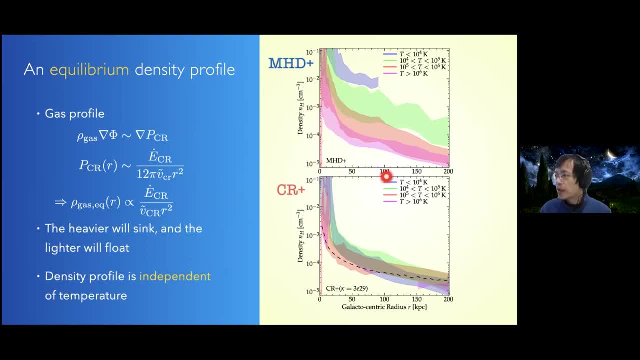 the gas density profile as a function of the radius, and different color means different phases of the gas And if there's no custom array, you can see that the cool gas must stay at a very large density And the hot gas must stay at a very low density. 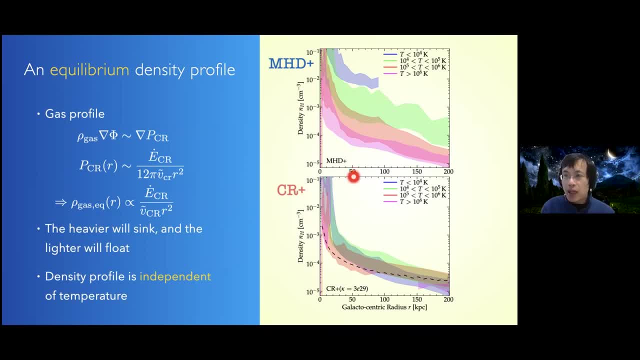 So that makes sense, right. Because if there's no custom array, different phase of gas must be in pressure equilibrium, right? So the hot gas must stay at a low density and the cool gas must stay at a high density. But now, with custom array, you can find that. 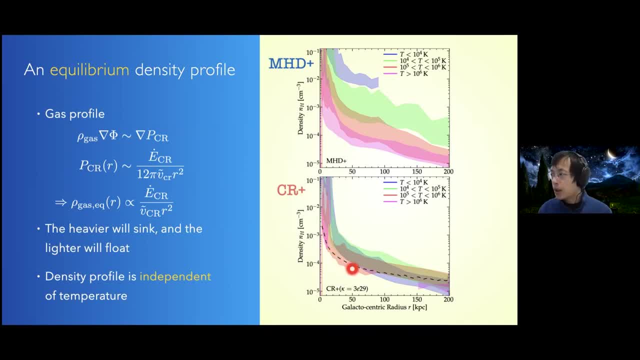 no matter the gas is cool or hot, it always stay at a very similar density And the dashed lines is our analytical solution. You can find that. so our simulation will meet this analytical solution very well And that will lead to a very important implication. 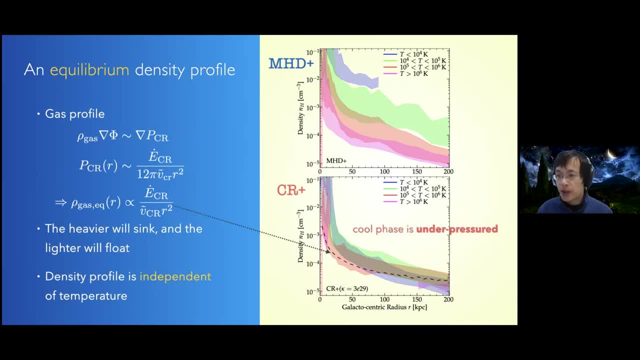 that is, the cool phase, must be under pressure. right, We have different phase of gas, they have different temperatures, but they have the same density. Then the cool gas. the pressure of the cool gas must be smaller than the pressure of the hot gas. 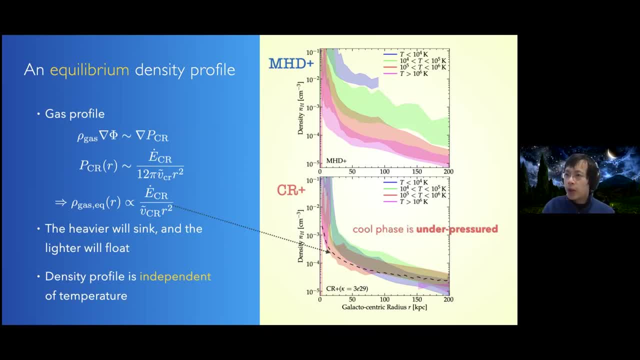 So that can help us understand why we can see a lot of unpressured cool gas in a CGM. So maybe that's supported by the know some of pressure from the custom arrays. And now you might be wondering that if the gas are not in pressure equilibrium, 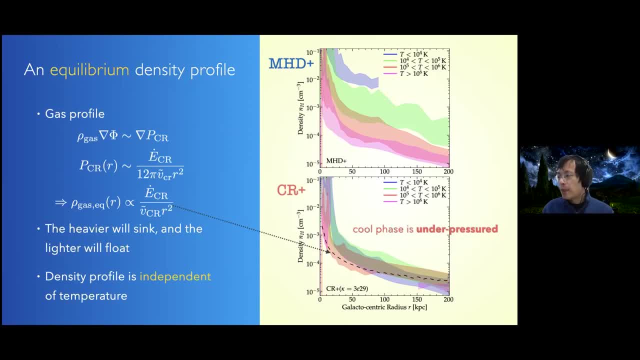 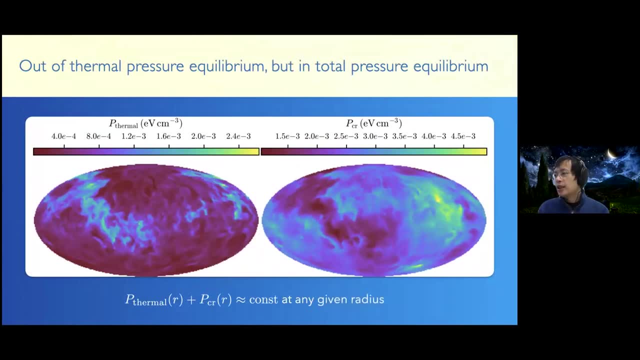 so why it can be stable. So here what we can do is we can make a cut of some fixed radii and expand it. So here we can see. I showed the map of the thermal pressure and as some fixed radii. 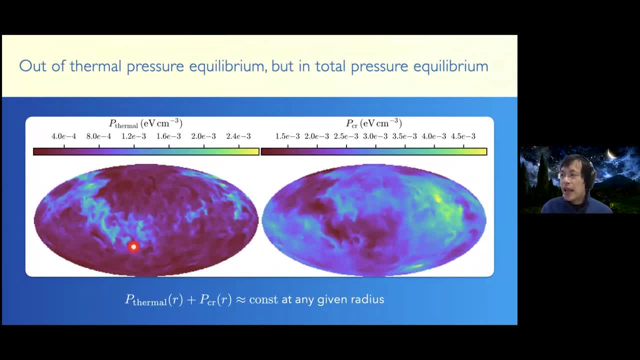 So it is relevant from the gravity And you can see that indeed, the gas are not in some pressure equilibrium at all. right, We have some high pressure here, We have some low pressure here, But if you look at the customer pressure, 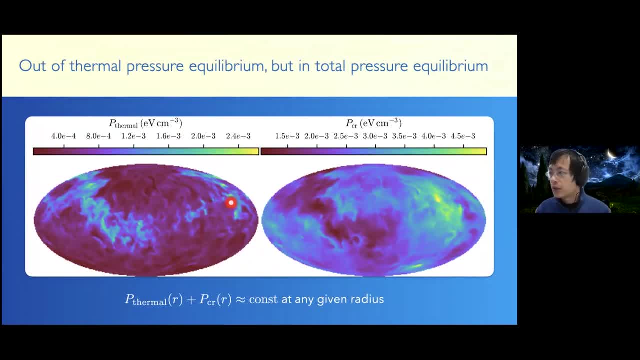 you can find that the two map are anti-correlated, right? We have some high pressure here, some pressure here. We have some low customer pressure here. So, in other words, the sum of the thermal pressure and the customer pressure at a given radii is a constant. 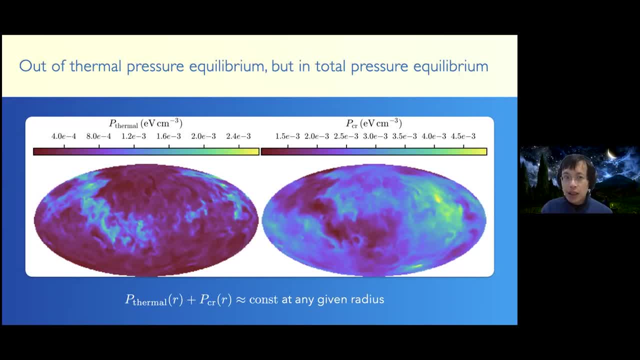 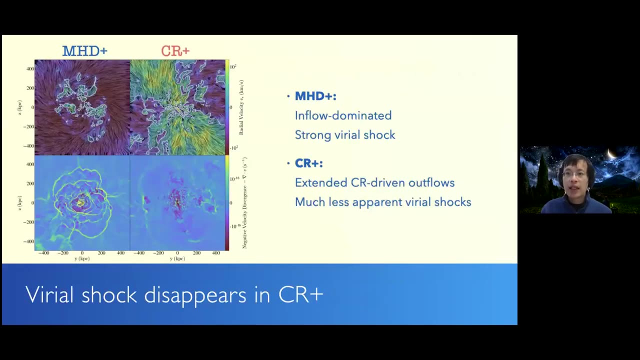 which means that although the gas are out of thermal pressure equilibrium, but they're in total pressure equilibrium if you bring customer pressure into consideration. And also we found that the kinematics of the CGM is great. It's been modified by customer pressure. 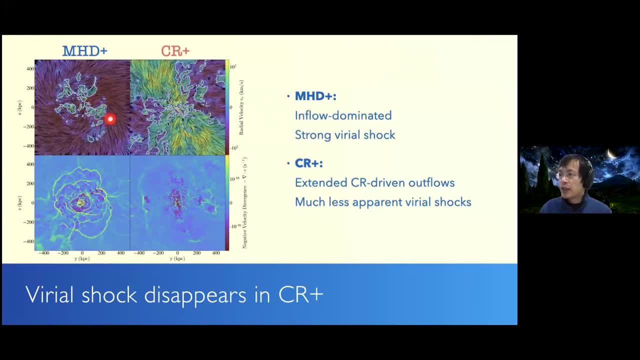 So here what I show is the top panel, So that is the velocity slice plot, And also on the bottom panel, so that is the native of the velocity divergence, So that shows the compressibility of the gas. You can find that if there's no customer. 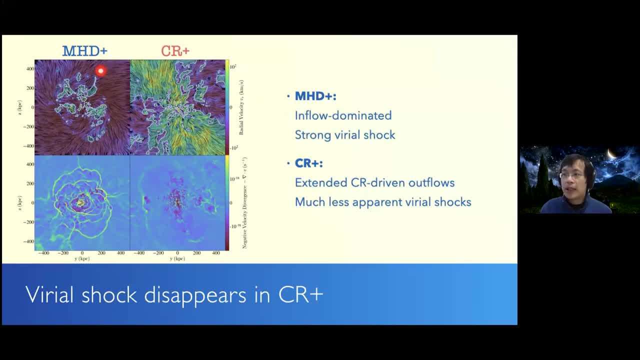 and the entire halo is dominated by inflow gas and it has a very strong, very strong right. There's a lot of chaff runs in the halo And with the customer rate you'll find that there's a very extended cell driven outflows in the biconcrete region. 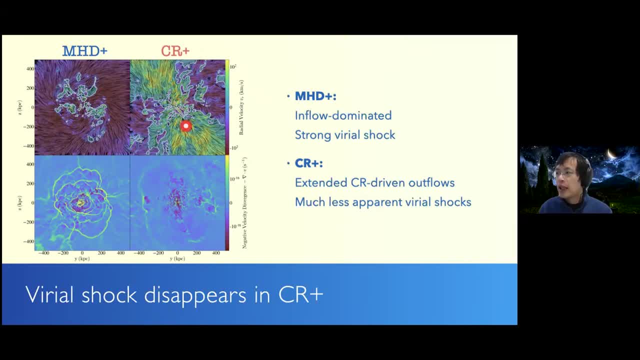 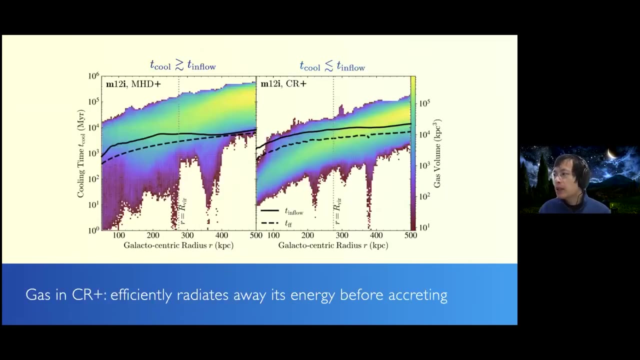 And the structure of the velocity transfer is totally different. And also you can find that there's no chaff run at all. So it seems that the real chaff disappears in the customer area. So why is that? So one way we can see that is, we can compare. 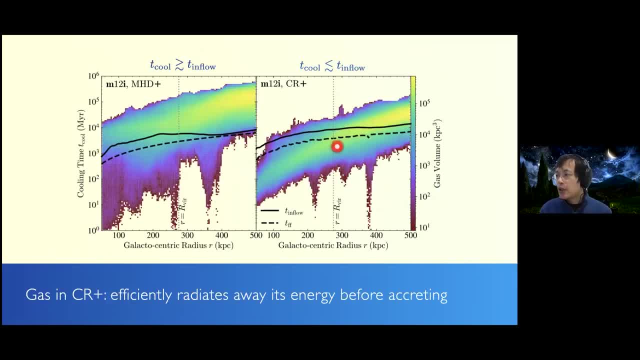 the cooling time and the inflow time. So here the color part is the distribution of the gas cooling time And the black line is the inflow time of the gas. You can find that with that customer rate and most of the gas for most of the gas, 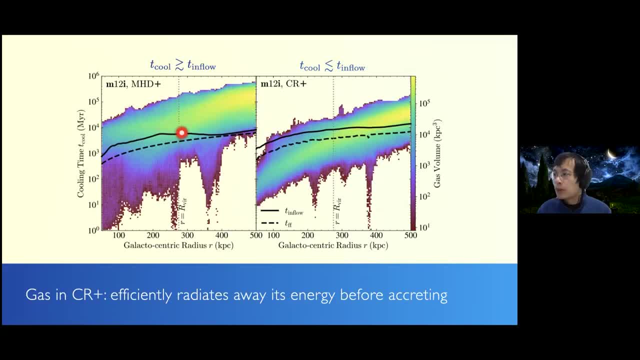 the cooling time is larger or comparable with the inflow time, But with customer pressure- most of the gas- the cooling time will become shorter than the inflow time. Therefore, if the halo is dominated by customer pressure, then the gas can efficiently radiate away its energy. 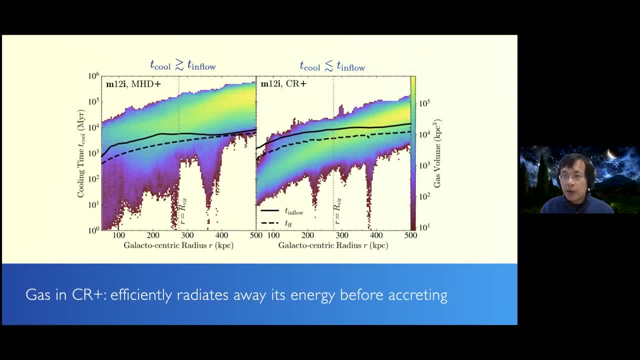 before accruing into the central galaxy. Therefore, there will not be enough thermal pressure to support a stable shock front. Therefore there's no shock at all, right, So that is a huge difference with you know, with that, And now with customer rate. 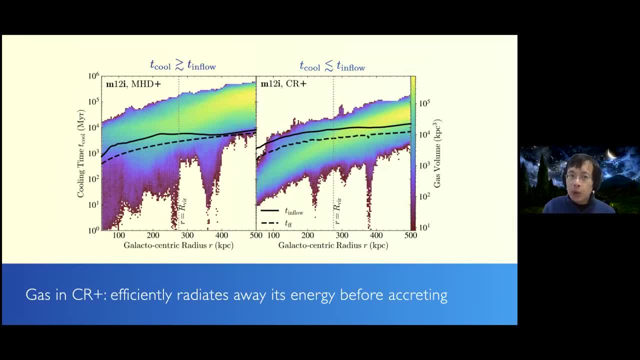 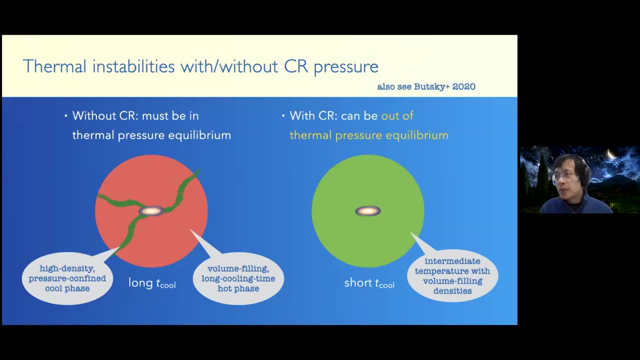 And you might be wondering so why the cooling time is so different with or without customer rate. Then we can look at the thermal disabilities, because the thermal disabilities behavior are totally different with and without customer rate. If there's no customer pressure, we know that different phase of gas. 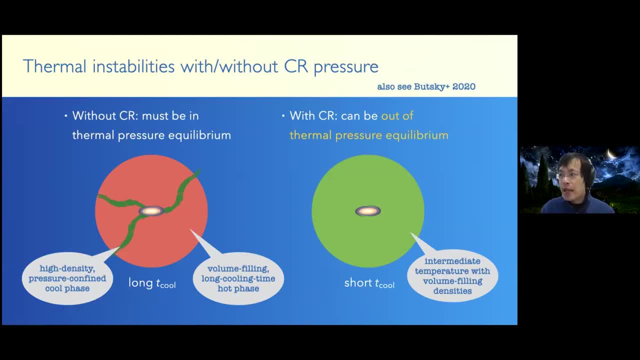 there must be in thermal pressure equilibrium right. Then the cool gas must be pressure constant right, pressure confined to a very small volume and the rest of the space must be filled with the very volume filling long cooling time, hot space. So the entire system will have a very long cooling time. 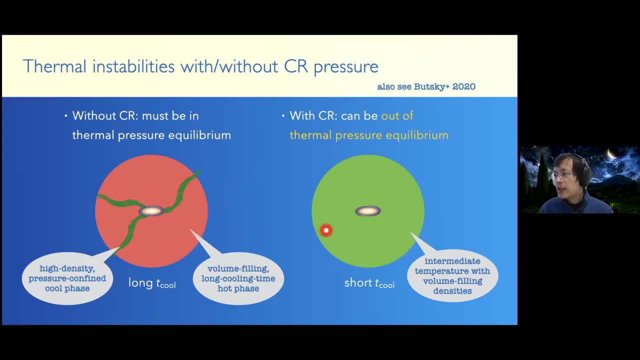 But if we include constant rays we can find that the entire gas halo can be out of thermal pressure, liquid metal right, And then the gas can cool down but still maintains a very diffused, very volume filling state. Therefore the system will have a very short cooling time. 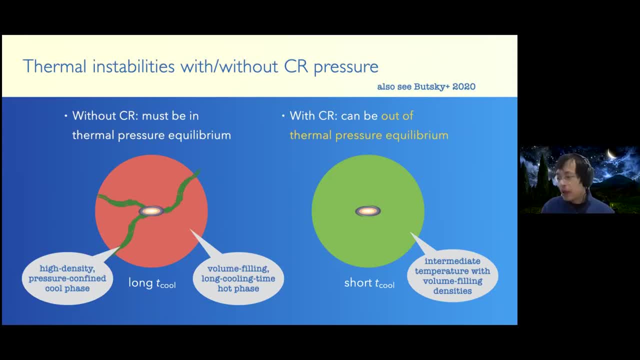 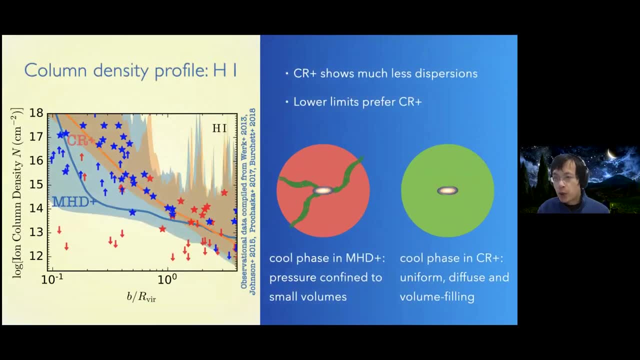 And with that we can better understand about our observations. So here I show the column density profile of H1, and the blue curve is our MHTD one and the orange curve is our Cosmere one, and the stars and arrows are from observation data. 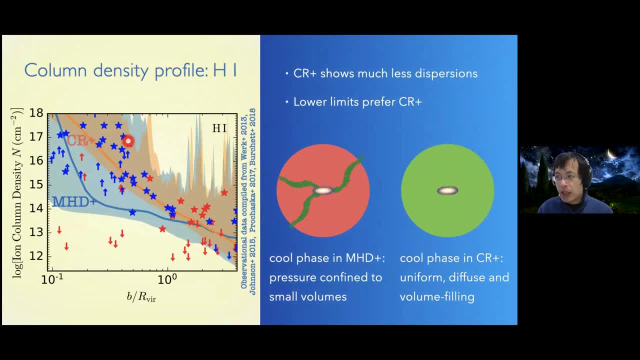 And you can find that the biggest difference between the MHTD one and the CETA one come from here, this part right. So it's that no constant ray. it's a large scattering here and it has a very low lower limit. 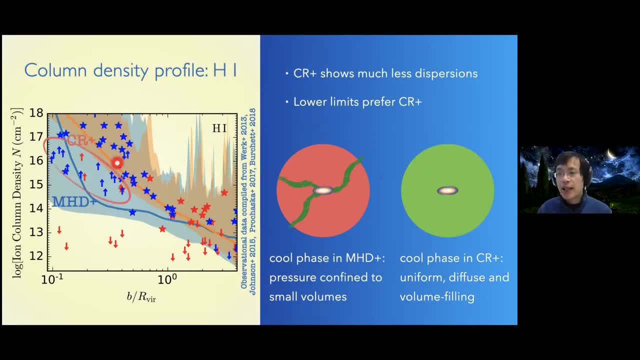 but with constant ray the scattering is much less and it has a very high lower limit. And if you look at the the upward arrows here, so that is the observational low limit. So I will say that maybe observation will prefer our Cosmere one. 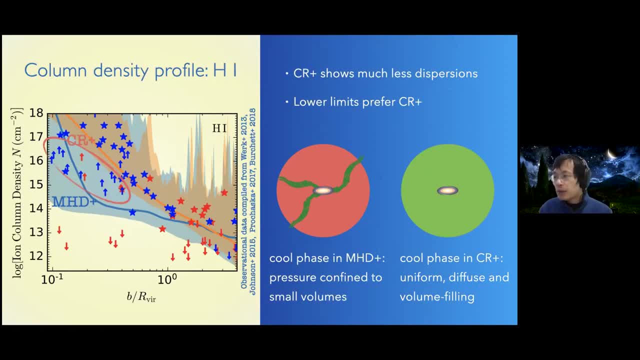 So why is that? As I mentioned before, so if there's no Cosmere, so the cool gas must maintain pressure equilibrium with the hot phase, then it must be pressure confined into very small region, right? So this is the picture, And if you shoot one side line, 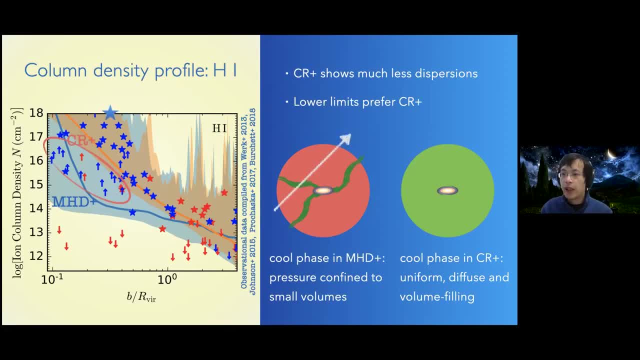 it might penetrate some cool gas, will give you very high, will give you a very large value And maybe some side line will penetrate no cool gas at all and that will give you a very low limit. So therefore, if there's no Cosmere, 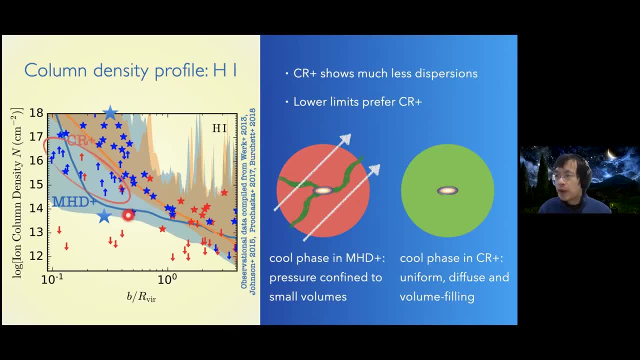 there will be a very large scatter And also you will have a very low, low limit. But now with Cosmere we know that the gas can be out of pressure equilibrium, so it can maintain the cool gas, can maintain the hot phase of the heat. 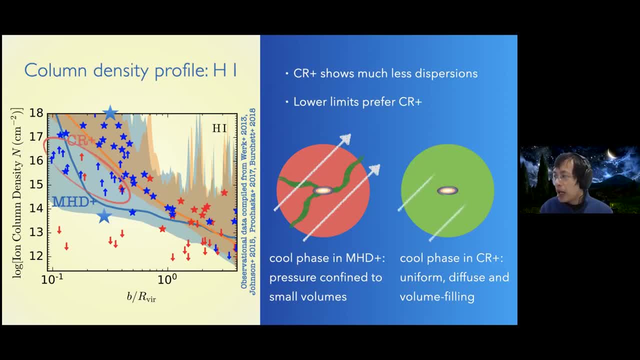 a very volume filling very uniform face. So no matter how you draw the sight lines, they always give you very similar value. So I would say the profile of the H1 or the scattering or the low limit of H1 will tell you or indicate what is the status of the cool gas in the CGM. 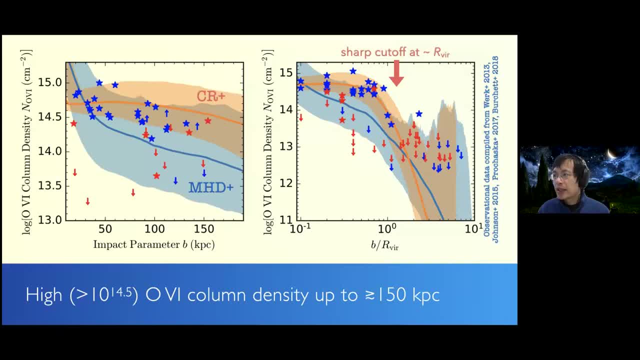 And also we can look at. what we care about is the O6. Again, the orange value, or the orange line, is our CR1 and the blue value is our NHG1. So it's very clear that our CR1 will fit the observational data extremely well And you can maintain a very high O6 density up to 150 kiloparsec away. 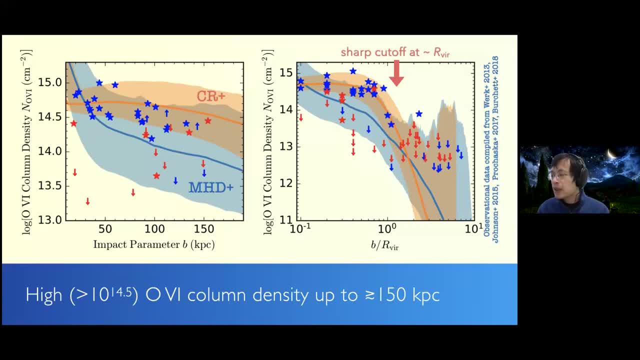 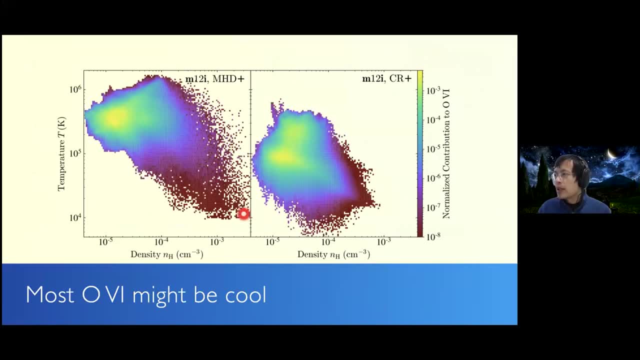 So that is a very exciting thing. And why is that So? here we can look at the O6 contribution as a function of H1. Density and temperature And you can find that if there is no carcimerase, most O6 come from the warm hot phase. So that is mostly come from the collision ionization. But with 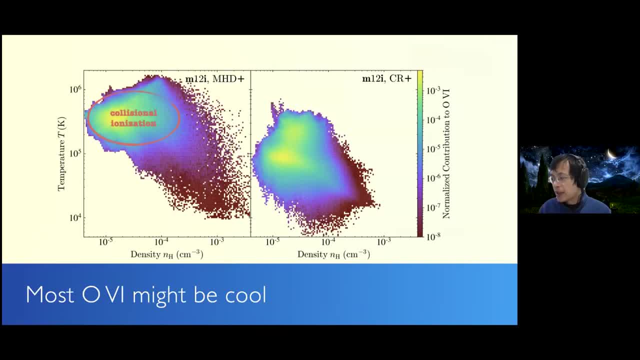 carcimerase you can find that most of O6 come from the diffused low temperature gas, So that is mostly from the photon ionization. This is because the carcimerase can maintain, can make the gas diffuse and volume filling So that can be very easily photon ionized. 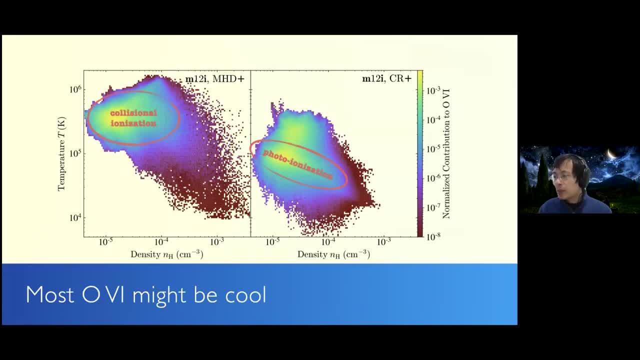 And that can also help us understand why the profile of O6 is pretty flat, Because if you go to the very large radii, although the total gas number, density drops, but the efficiency of the photon ionization will increase. So therefore, even at very large radii, 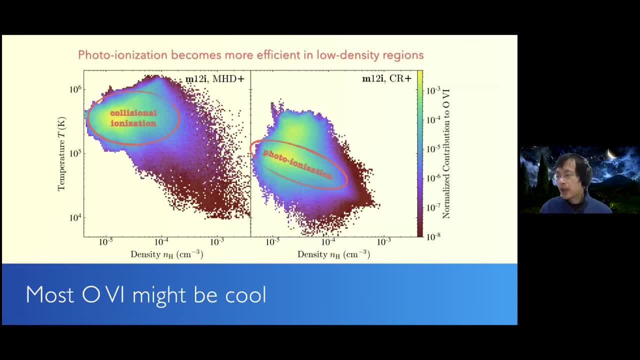 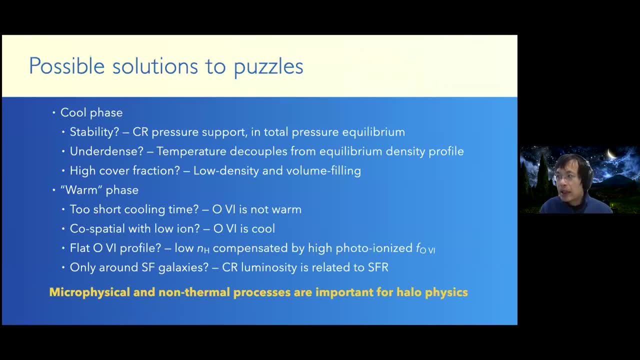 you can still see a lot of photonized O6. So the summary is that maybe if we include the non-soluble carcinoma impact, we can perhaps understand the problem in the CGM For the cool gas. so why is it stable? 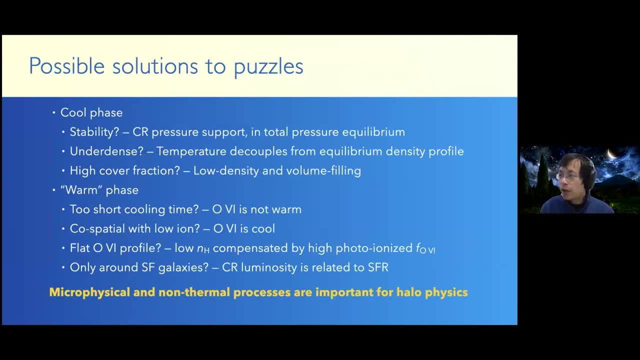 Why is it dense And why it has a very large cure fraction? Maybe because the cool gas is supported by customer pressure. then it does not care about the gas temperature anymore And for the warm gas, so why it can be there, given its very short cooling time. 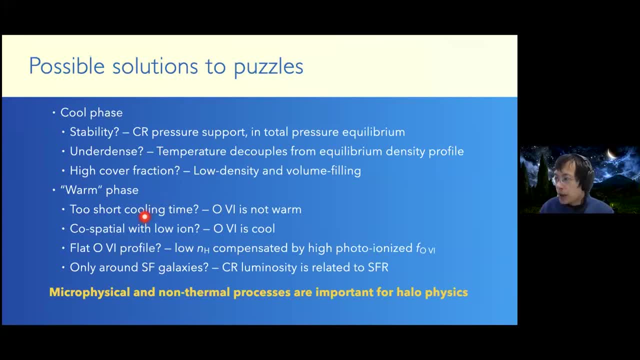 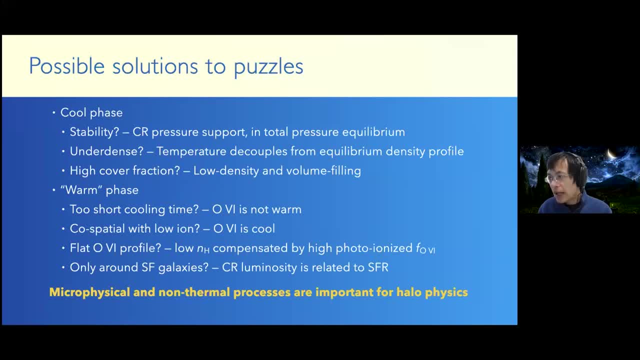 gas, right, So it's actually not warm and actually it's cool. And also why you can only see warm gas- a so-called warm gas- around styrofoam gases, because we know that the C-aluminosity is related to our styrofoam rate, right? So if there's no, 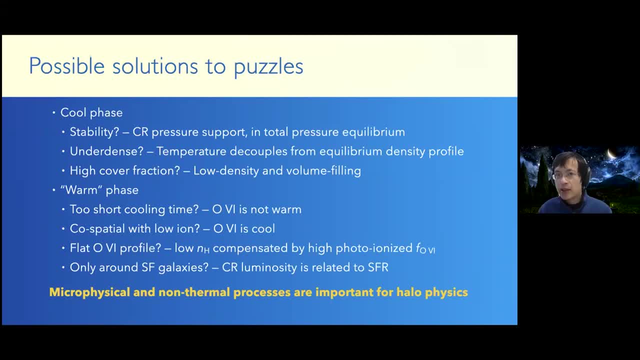 styrofoam emission, there'll be very little constant rate of luminosity, so there will be no C-al supported halo. So I think the bottom line is that I think the micro-physical, the non-summar processes, such as magnetic fields and constant rays and turbulence and so on, 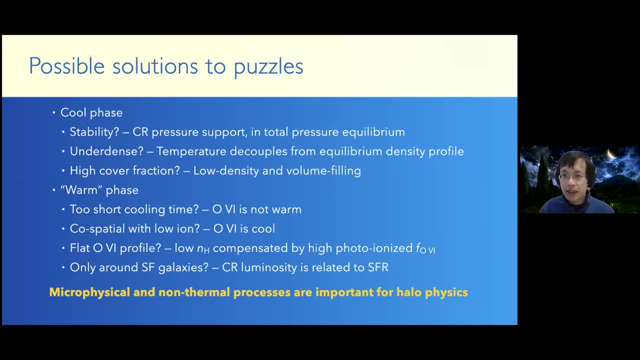 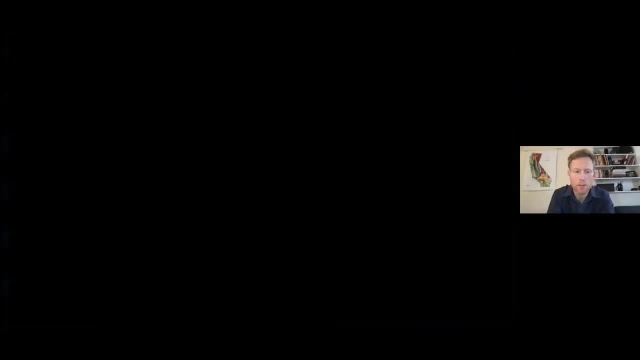 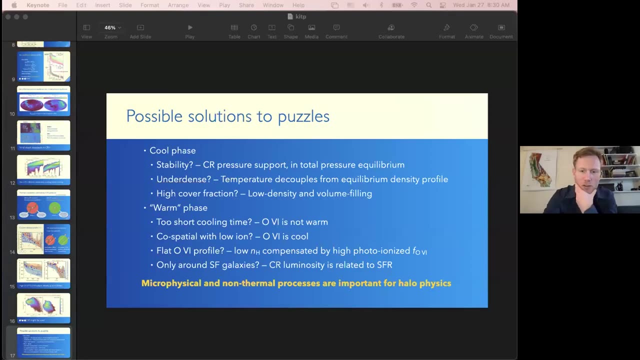 are very important for us to understand the physics of gas halo. So that's all and thank you for your attention. Thank you, Suqing. It was a very clear explanation of the potential impact. Thank you, Suqing. I think that's a very clear explanation of the potential impact of cosmic. 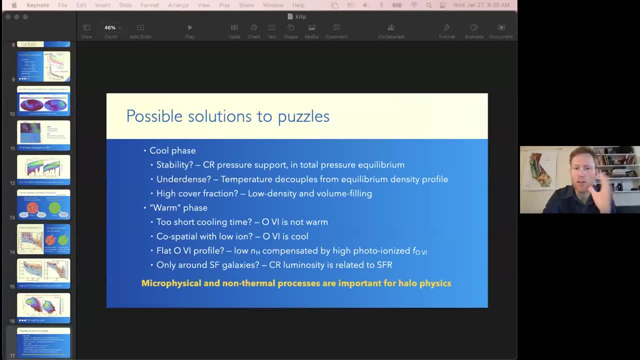 rays on the CGM and on the halo. We already yeah. so, as I mentioned, just for everyone's reference, we'll take like 10 minutes or so of discussion in here, and then I encourage people who are interested in continuing the discussion to go into the appropriately themed breakout room. 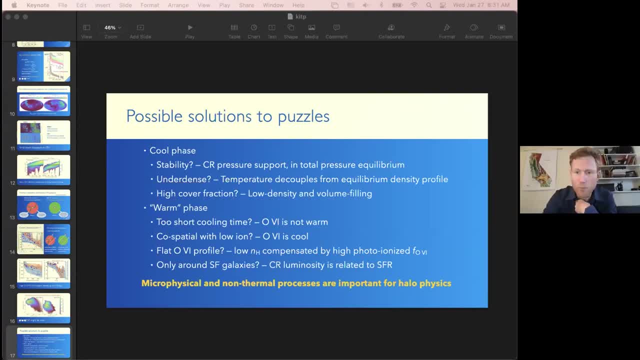 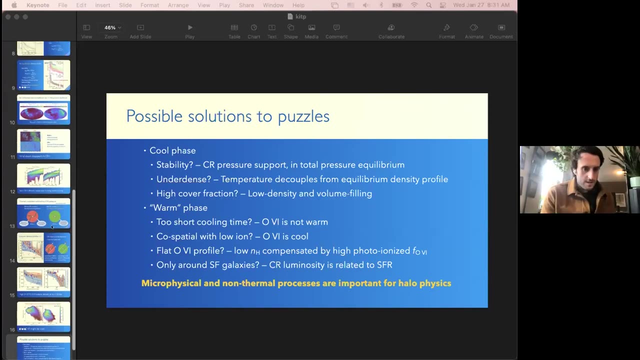 before we get started with Yuan Li's turbulence discussion. But I think the first person who had their hand raised was Drummond, Would you Thanks? Thanks, Suqing. Very clear, nice presentation as usual. Could you go back to that slide 14? your cursor is floating over. 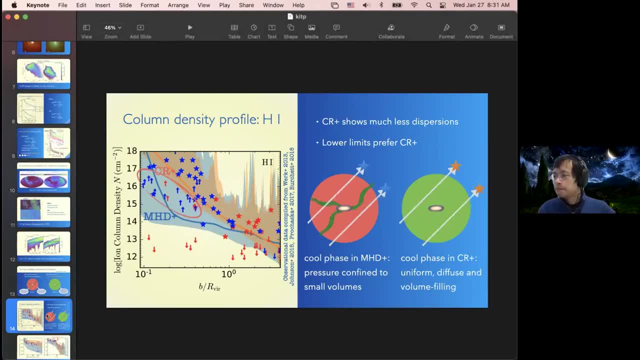 Yes here, Yeah. so when I look at H1 absorption in papers by all of the wonderful observers on this talk, the H1 absorption is coming from very narrow or. you know, forget H1,. you know magnesium 2, silicon 2, tracing, that sort of. 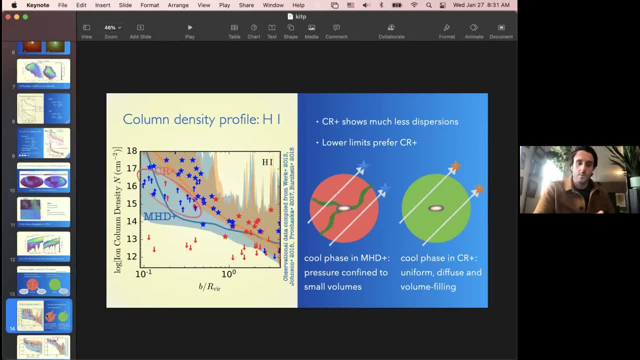 you know, cool 10 to the 4 Kelvin gas. It comes from very narrow absorption lines And I know Cameron was a co-author on this paper with you, so I was wondering if you could say anything about the line widths of the low ions in these two scenarios and if the CR plus halo. 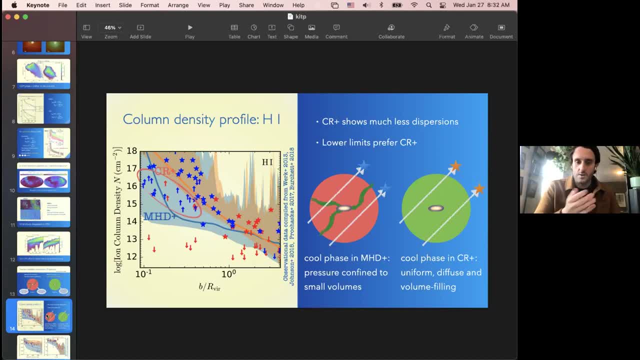 line widths are actually consistent, as you're showing the. you know, the integrated ion column densities are. Yeah, so that is a good question. So, actually, it's indeed so. our future plan is we can probe the line widths by looking at the synthetic CR spectra from some of the patients. 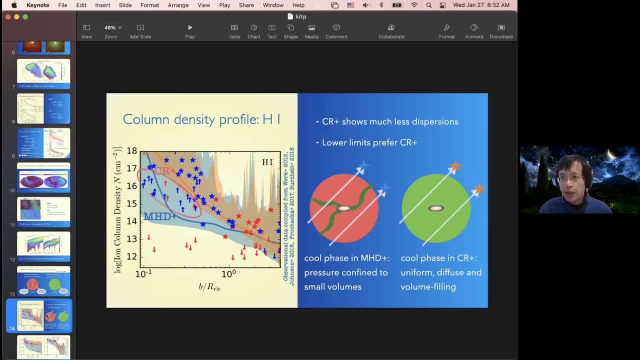 But now I do not have a clear conclusion for that. But I think the total thing is that the main thing is that because if we look across the glucose strain and the cool will be volume filling, So it should correspond to a very large coherent length scale. right, 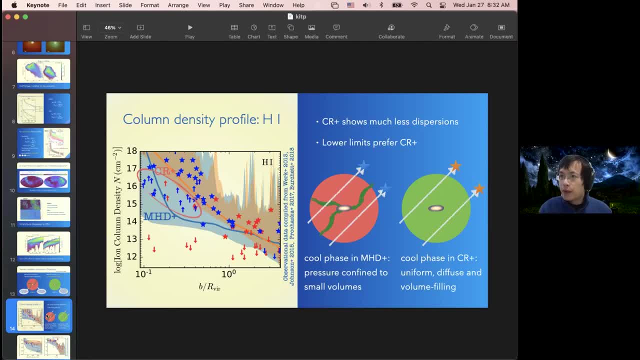 So if that is true, we should see a lot of motions that might be coherent at some length scale. So that will definitely impact our synthetic spectra of the production lines. So yeah, I think you might see some very broad, some very broad ions. 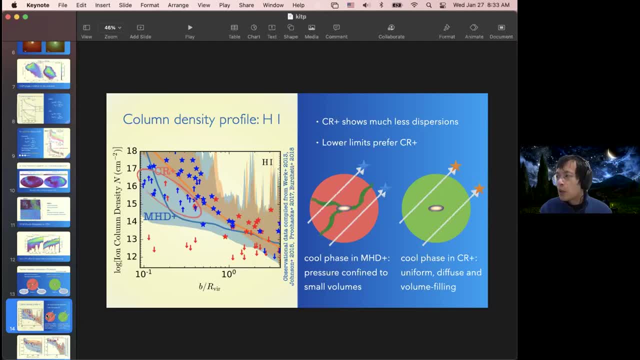 Yeah, but also it is kind of depends on: so what is the coherent length scale? So that is something we can. I cannot say for now for sure, but it definitely something I want to check in the future. Yeah, Thanks, Yeah, excellent question, And I think there are a lot of clear ways in which this can. 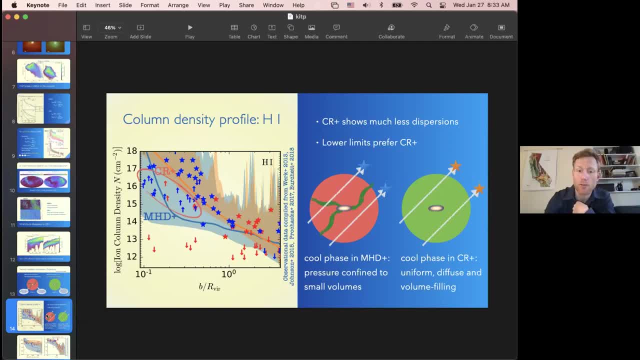 be tested and put constraints on by the observations on just what the strength is. So it's it's future work. I think, Yeah, All right. Next question from Yong: Yes, Thank you, Thank you. So I think that's a really great talk. So yesterday Pam mentioned: 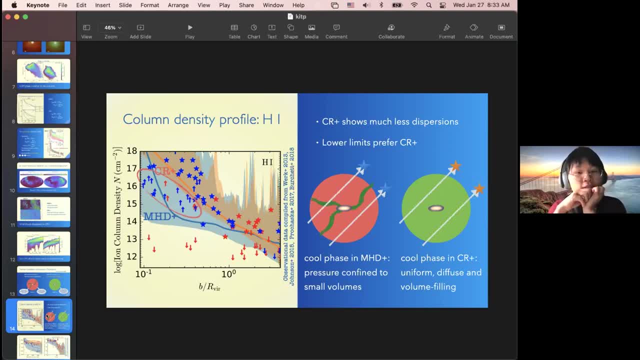 in ISM this energy partition between the gas pressure and the magnetic field and turbulence and whatever everything's in it. Yes, And then he mentioned in the CGM actually gas pressure dominates. So I was wondering, in your model right now, when you pump a lot of cosmic rates, 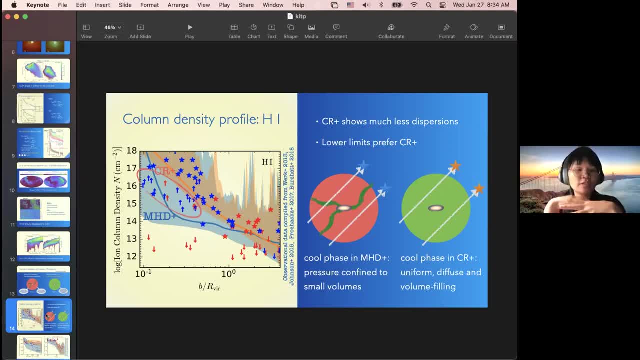 Yes, into it and boost the cosmic repro Zhanchen. how does that energy equal partition scenario look like? ah, I see, And related to that question, and so you assume that there is 10% of the supernatural energy goes into the cosmic rate, And how does that? 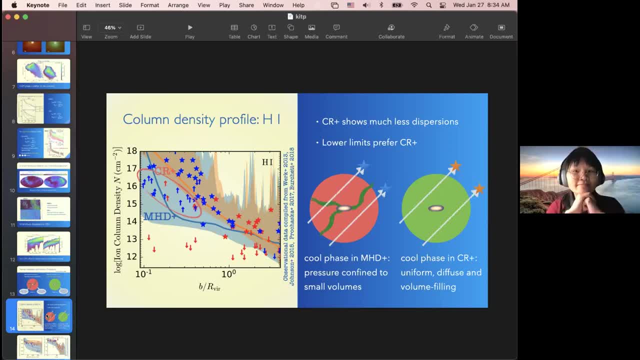 affect the overall outcomes of the CGM. Yeah, Great question. So if you come to the words of because of the so-called equal partition, So I'm not a, so I'm doing not like that вер tribute into it- What do you think about CGM otherwise? 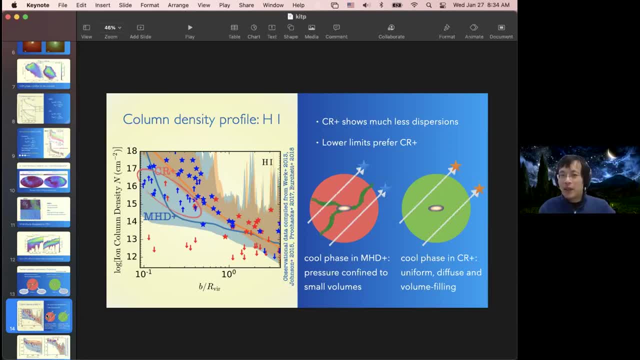 like that equal partition words very much. The reason is that. so when we say equal partition, we must understand what is the physics behind right. So, for example, you have some turbulent dynamo, We have. we say: we have equal partition. 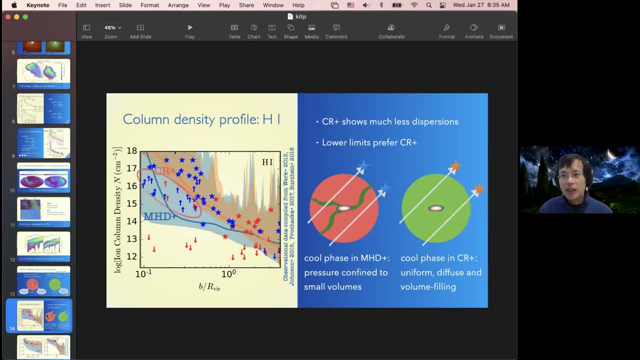 between the kinetic energy and the magnetic energy. So what you imply is that maybe there's some growth rate will be balanced by some damping rate. So that will give you the so-called equal partition right. But the equal partition is not a universal rule. 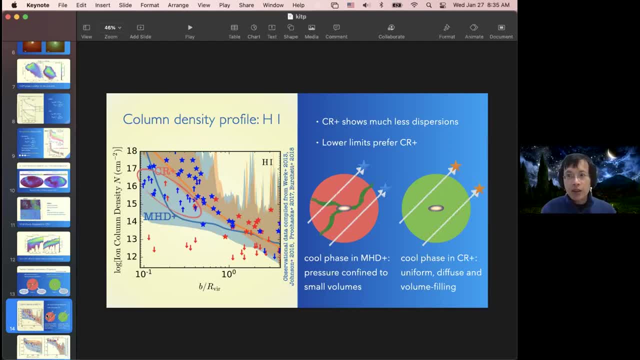 because we need to identify what is the physics behind. So what is really the balance of force between the two parts, right? So now, in our CGM case, the key thing is that is, the balancing is between the gravity and the pressure gradient of constant pressure, right? 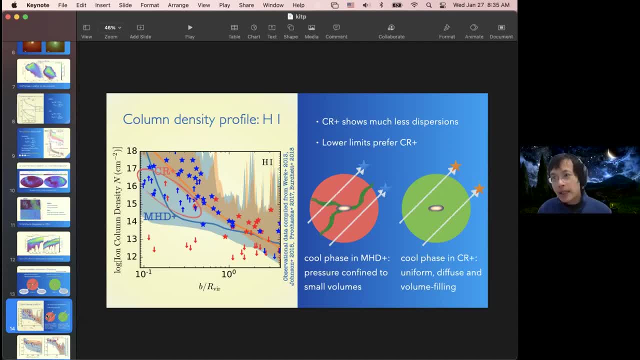 So that's this. two parts are comparable, So maybe equal partition between the thermal energy and the constant pressure might not hold right, Because of what is really balancing between these two is the constant energy and the gravitational potential. So I will not say that. 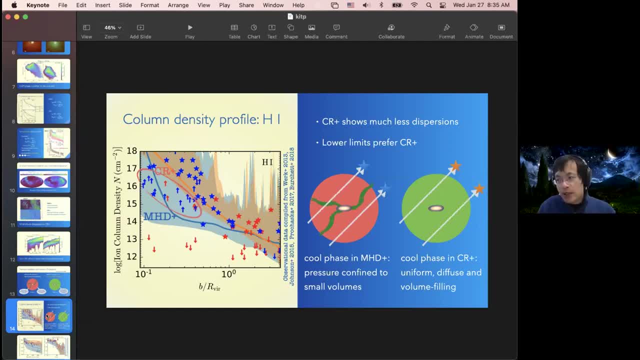 So I'll not think that. maybe the partition, So I would say that the equal partition might not be a good assumption in a CGM. But also I will say that if you want to consider the confinement and constant rate and how in that with you know. 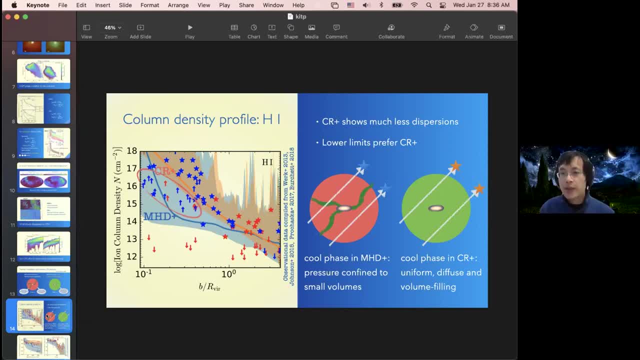 and how in that with you know, and how in that with you know, with the magnetic field, the very smart scale. So maybe there's some, there's still some balance over there. So maybe you can say some competition from that side. 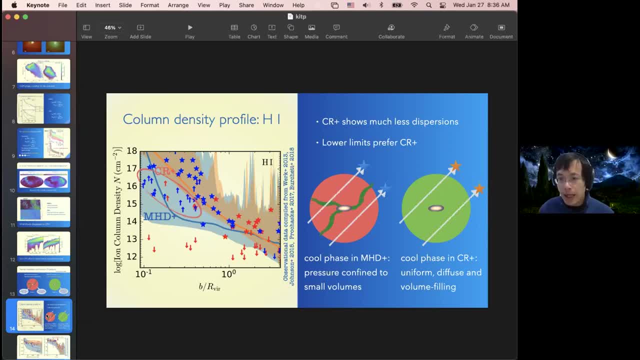 but on a global scale. so we did not anticipate equal partition between the thermal energy and the constant energy. And come to your second question. Yes, the star formation rate is really important because our model assumes that that's 10% of the solar energy would go to constant rate. 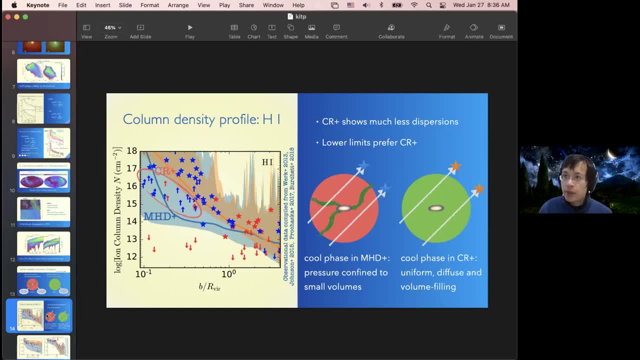 So that is based on, I'll not say solid, but it's a widely accepted number of 10% And also so that is what I can say right now. So I'll say, if you want to understand that better, so, indeed, how much. so what's the percentage? 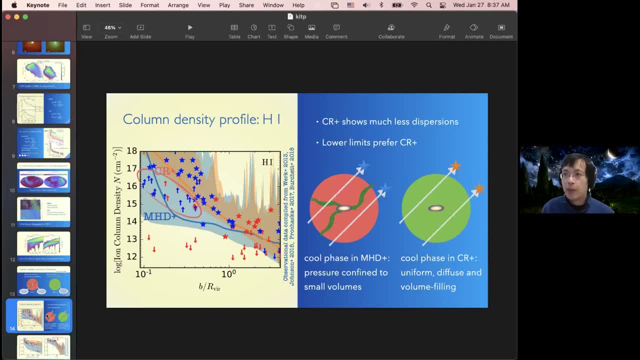 of the scourge or go to scourge. you need to do some more detailed study, So maybe the Parkinson's study to figure out the number, But 10% is at least a reasonable number for now. yeah, Okay, so we're bumping up on the time. 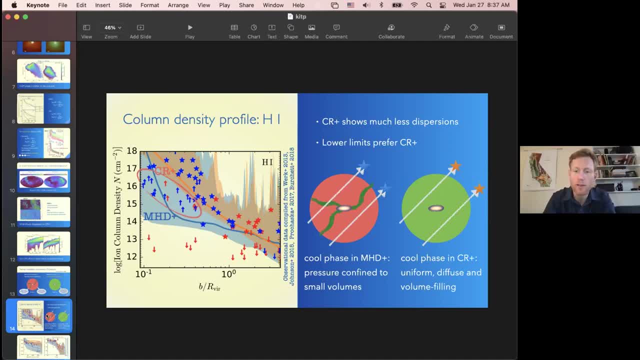 before we start our next tutorial by Yuan Li, So I invite. I know there are a number of hands raised. I'm sorry we didn't get to you. I invite everyone, including those who have their hands raised or people who are a little bit more hesitant to ask a question. 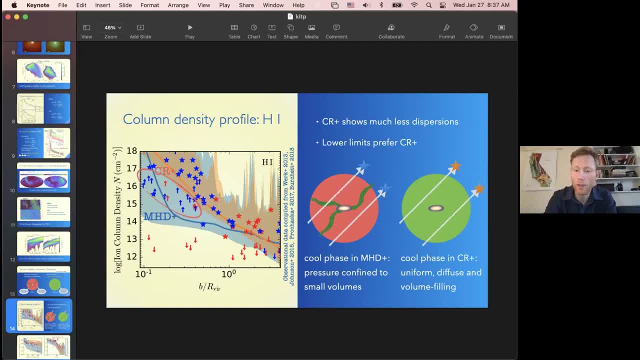 but want to stay on for this discussion, to go into the breakout room specified with cosmic rays, So Ching will also go there and be able to continue this discussion. We will start Yuan Li's tutorial at 8.40 in three minutes. 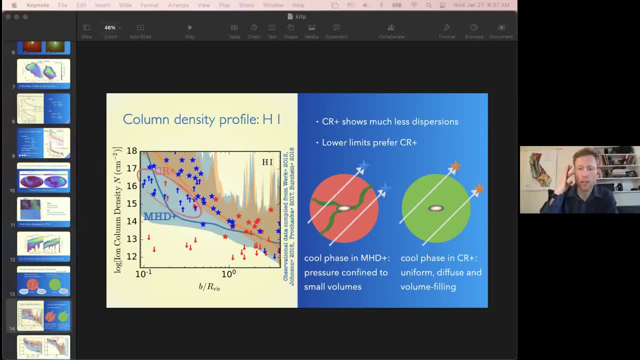 And then, if you guys want to come back from the other breakout room in the next bit, you can catch hers or catch Mateusz Ruszkowski's tutorial at 9.20, but I'll check in there and let you guys know when Mateusz is about to begin. Thank you.